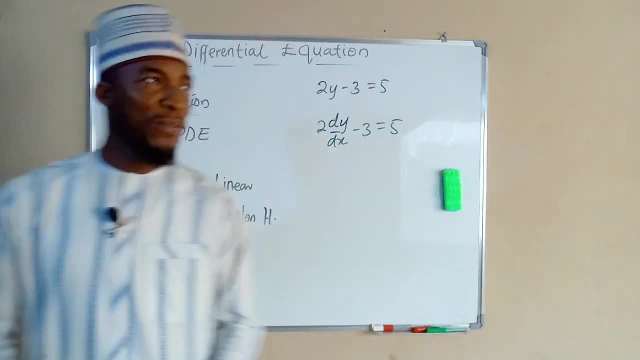 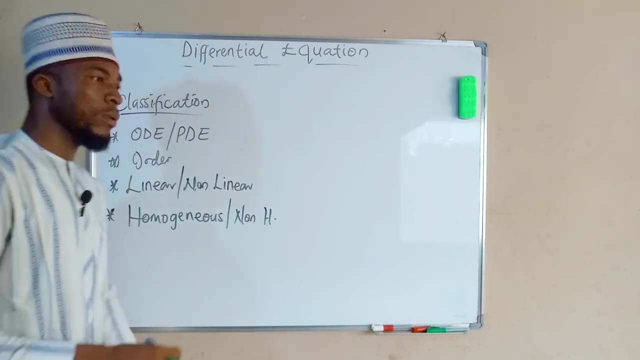 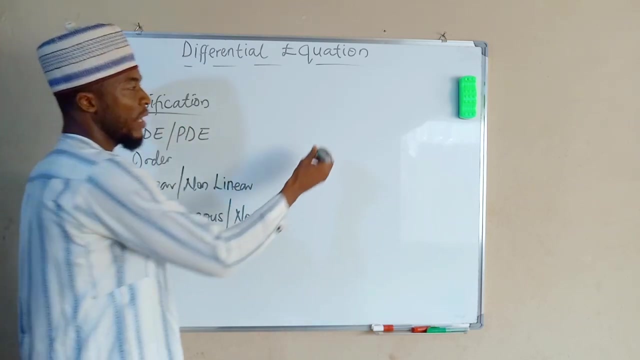 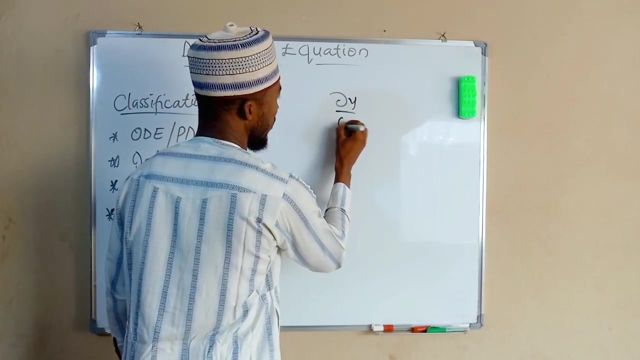 This is a differential equation. A differential equation may appear to be an ordinary differential equation or a partial differential equation. What differentiates the two is an ordinary differential equation. It does not contain partial derivatives, And partial derivatives are donated by delta notation. Maybe delta y over delta x. 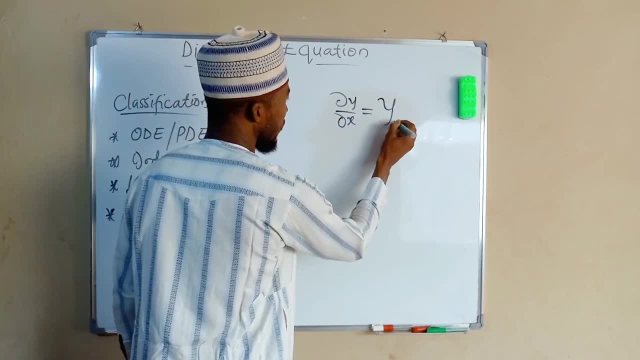 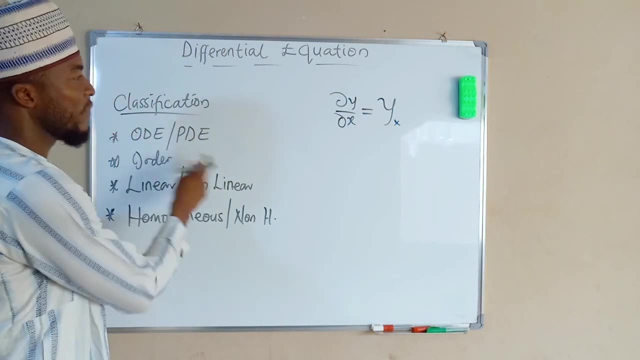 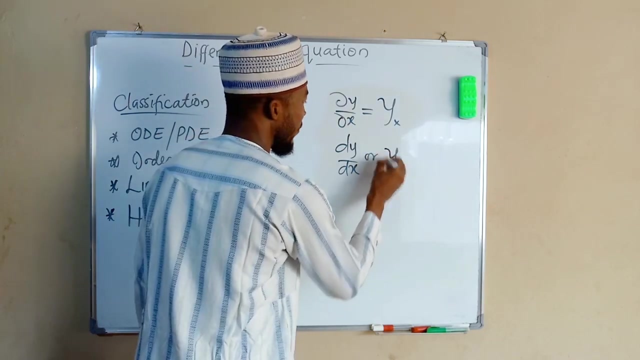 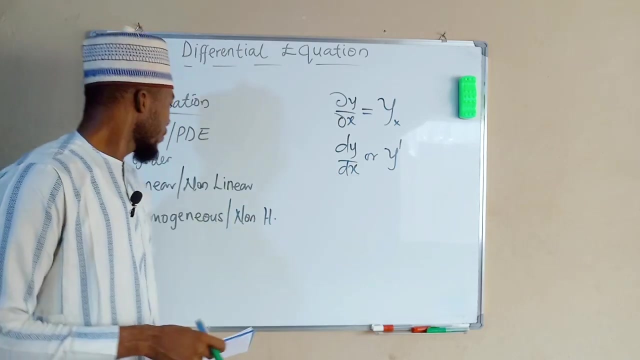 It can also be written in subscript form, which is y subscript x for first derivative, While ordinary differential equation is written like: dy over dx over y prime. This donates partial derivative, while this donates ordinary derivatives. Having done this, we can now see that the differential equation is written like this: 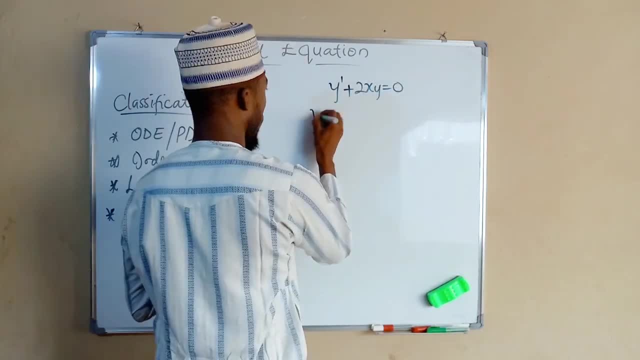 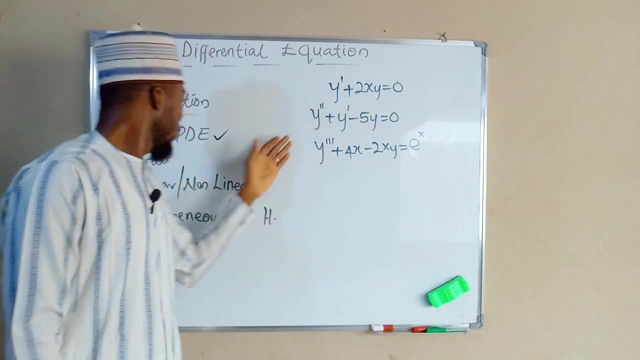 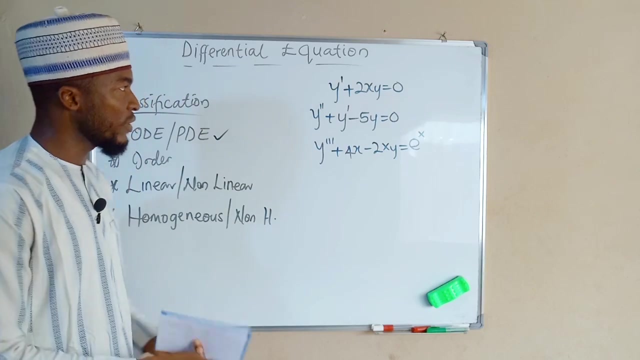 Having done this, we can now see that the differential equation is written like this: Having done this, let us move on to order. Here are some examples of differential equations. To find out the order of this differential equation, first of all you have to consider the highest degree of our derivative in that equation. 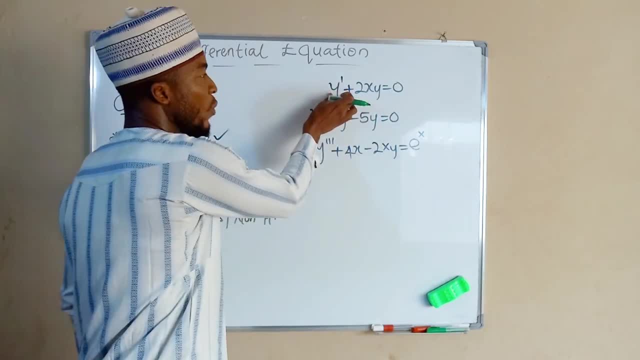 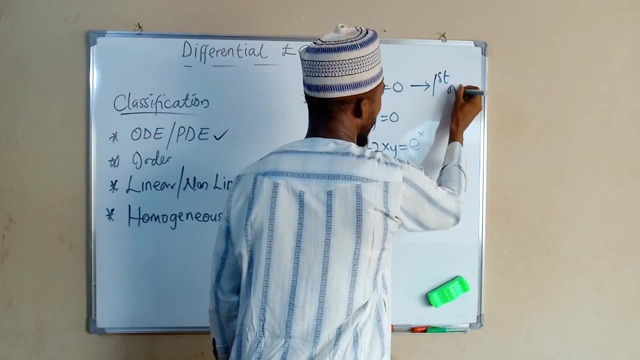 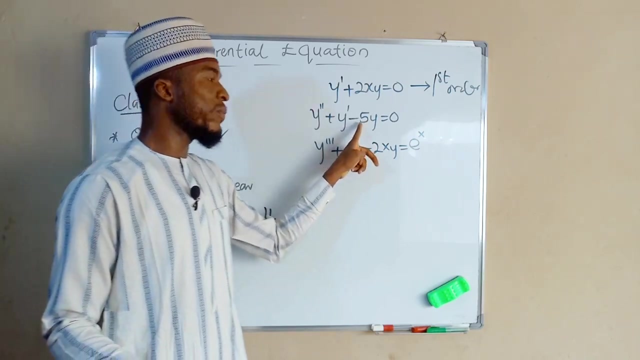 If you can see in this equation the highest degree, we have a first derivative. Therefore we say this is a partial differential equation of the first order. This is another differential equation: y prime prime plus y, prime minus 5y equals to 0.. 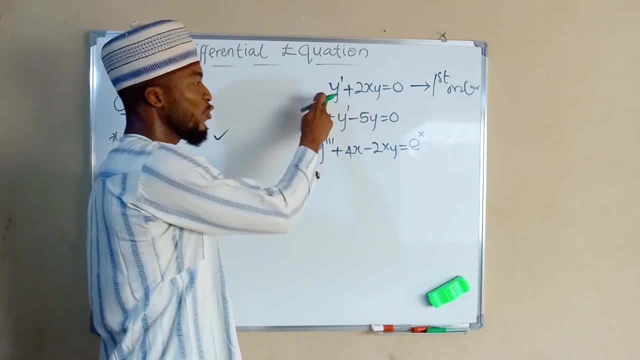 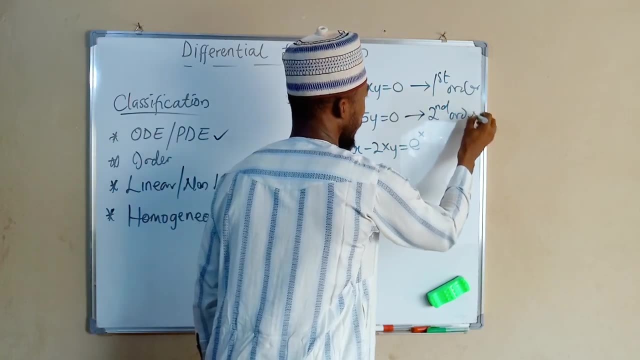 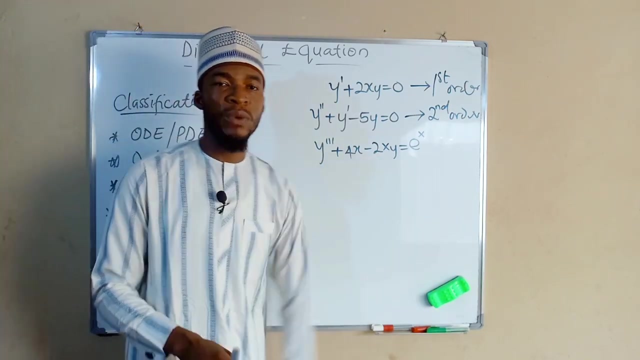 But the highest degree of our derivative there is 2.. This is second derivative, so we say this is second order. differential equation. And lastly, we have y prime, prime prime plus 4x minus 2xy equals to exponential x. So we say this is third order. 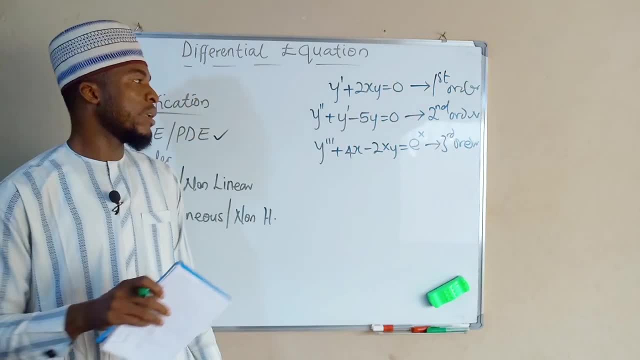 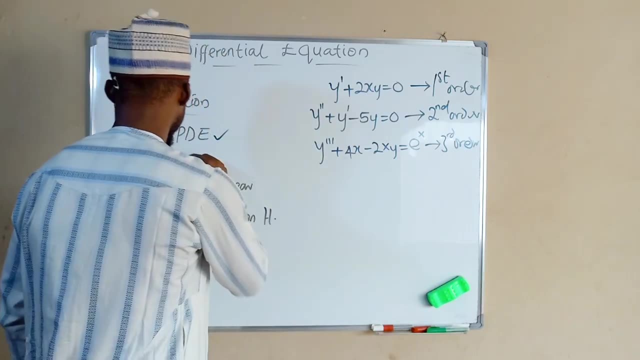 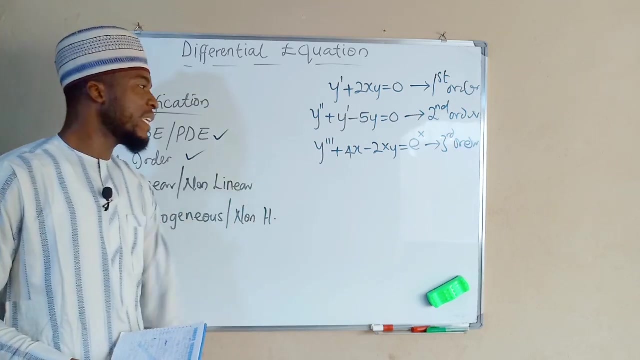 This is the third order differential equation in that order. So the highest degree of our derivative in differential equation determines the order of that differential equation. We are done with this. A differential equation can also appear to be linear or nonlinear. I think to have a clear understanding of their differences. 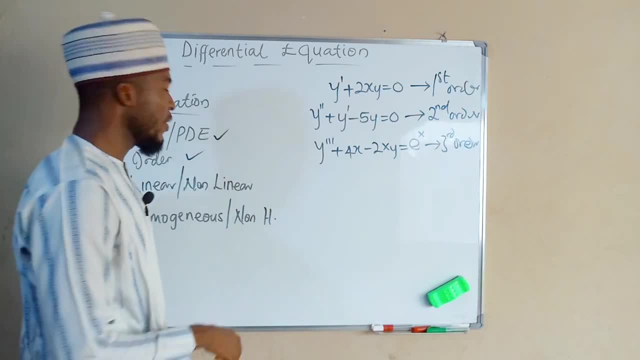 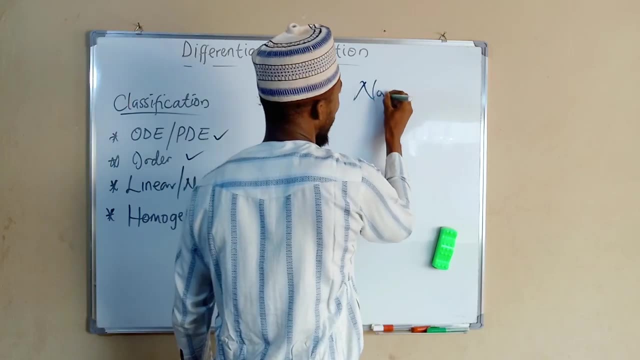 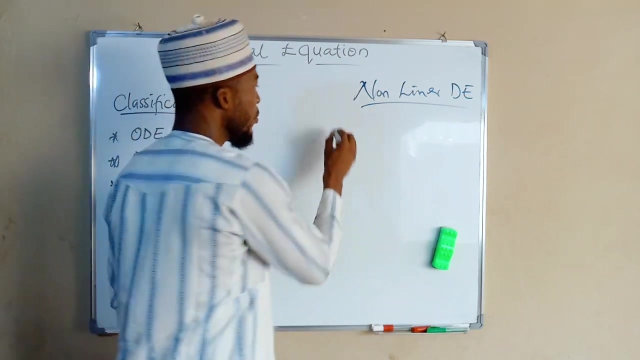 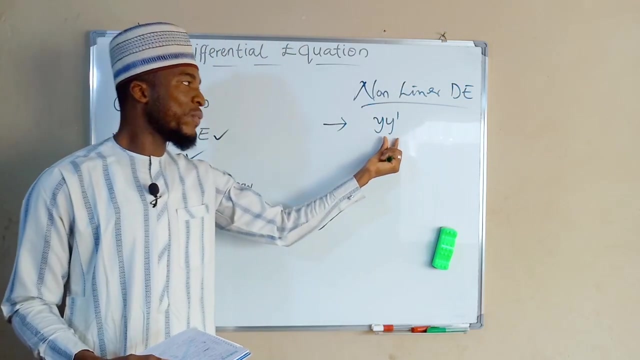 let me highlight the characteristics of this nonlinear differential equation. All other characteristics will fall under linear differential equation. Nonlinear differential equation. A nonlinear differential equation, you may have a term in the form of y, y prime. Whenever the coefficient of our derivative is y, that differential equation is nonlinear. 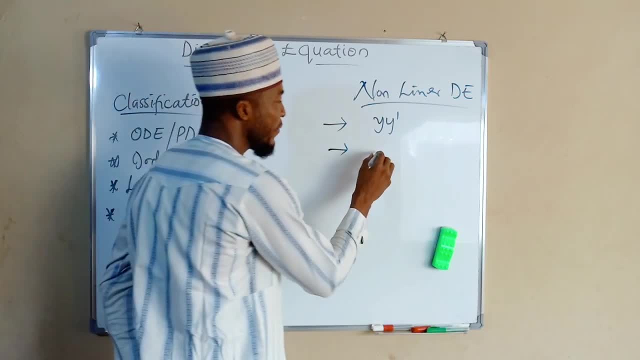 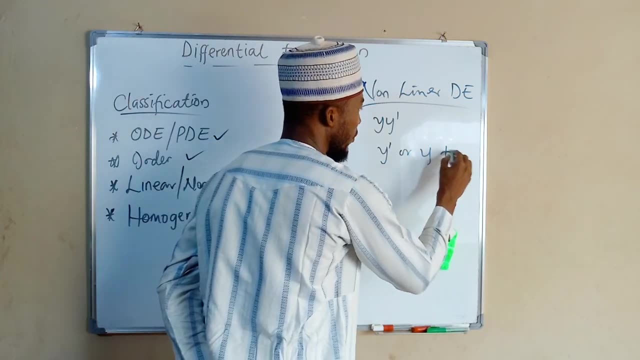 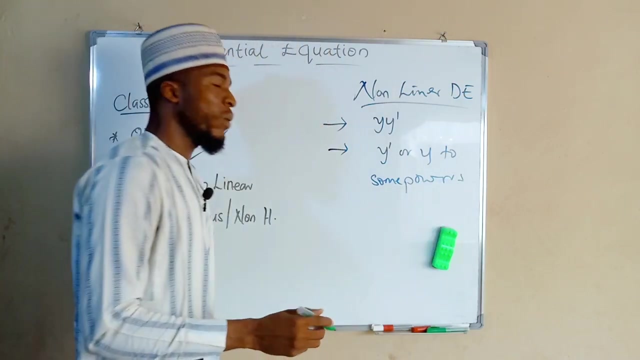 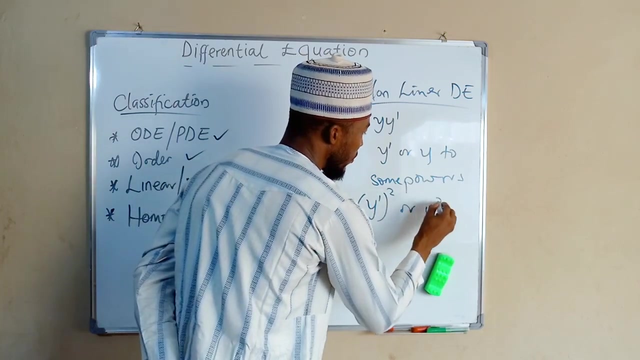 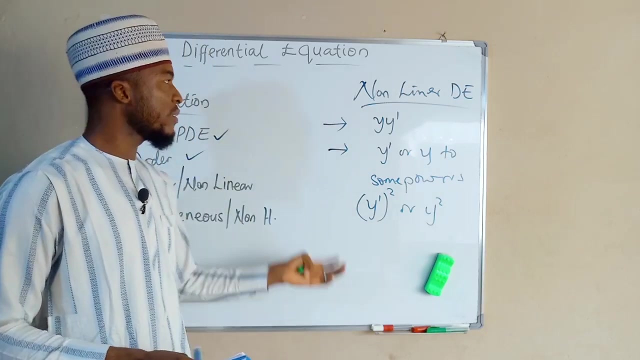 And secondly, y prime o Y to some powers to some powers. Whenever you see our derivative like Y prime to maybe second power or Y to the second power, that is nonlinear differential equation. Otherwise we are going to categorize it under linear. 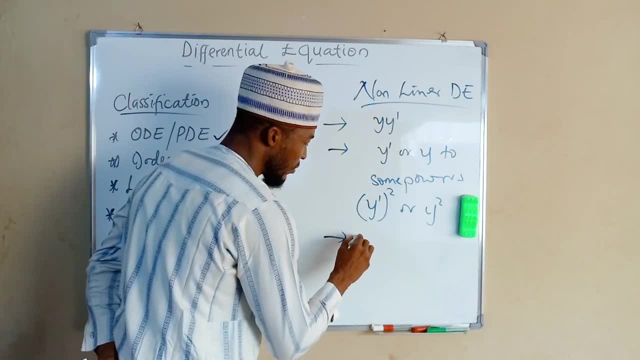 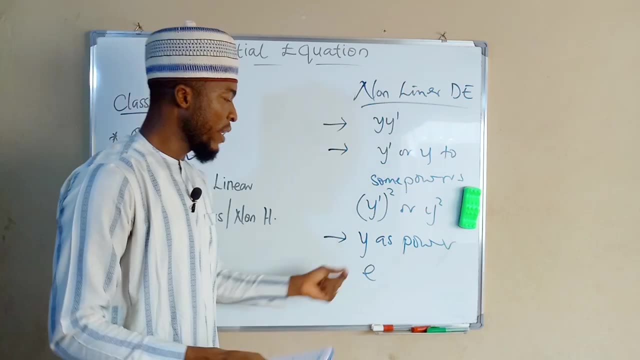 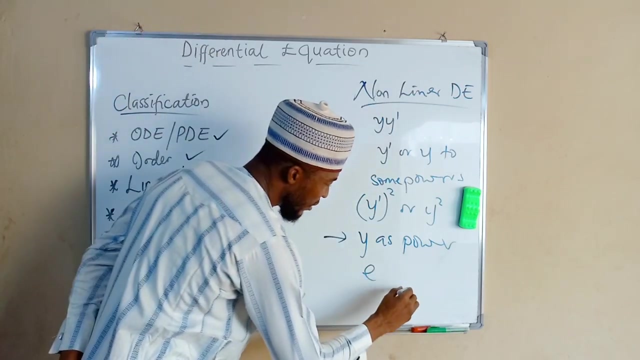 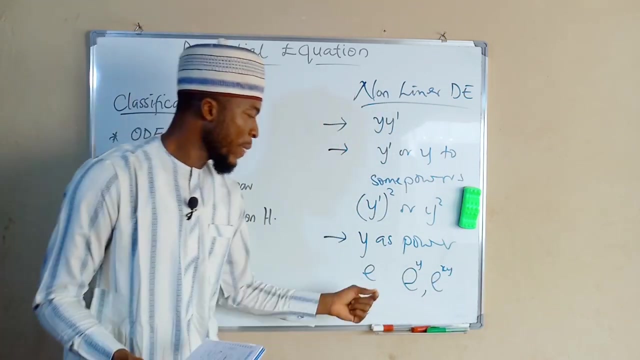 differential equation Y as power of E. In linear differential equation, E cannot take power of Y. so therefore, in nonlinear you can see exponential Y, exponential XY and so on and so forth, but in nonlinear it can only take power of X. Another characteristic scenario that we are going to discuss today is that we 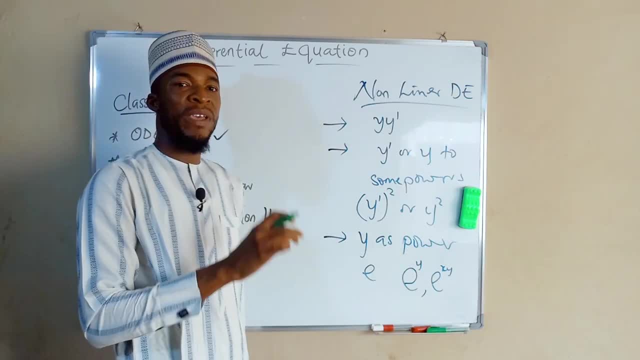 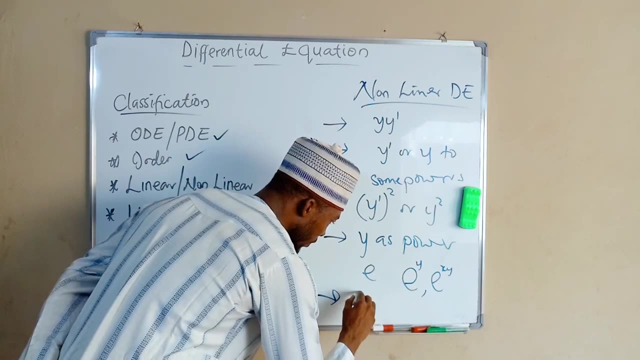 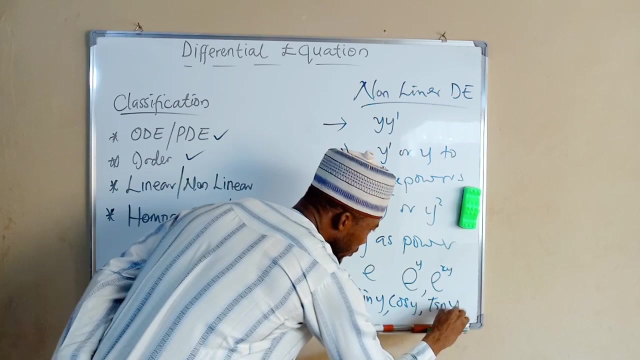 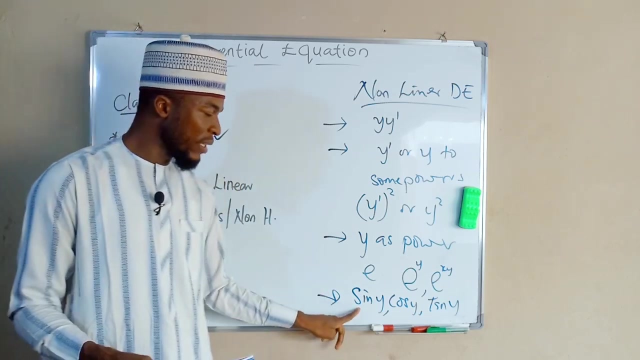 under nonlinear differential equation is that y can appear to be the argument for our trig function, like maybe sine y cos y or tan y and so on and so forth. In nonlinear differential equation we may have this function, but in linear differential equation you will never see sine y cos y, tan y and other trig. 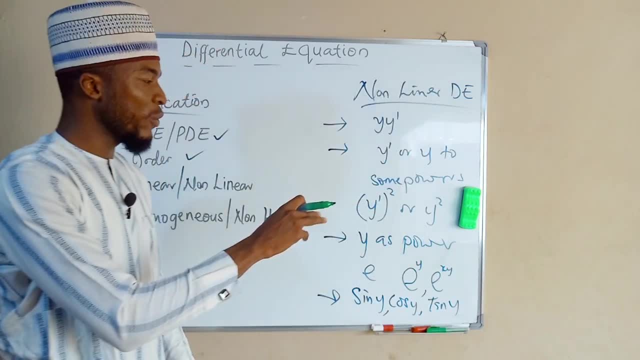 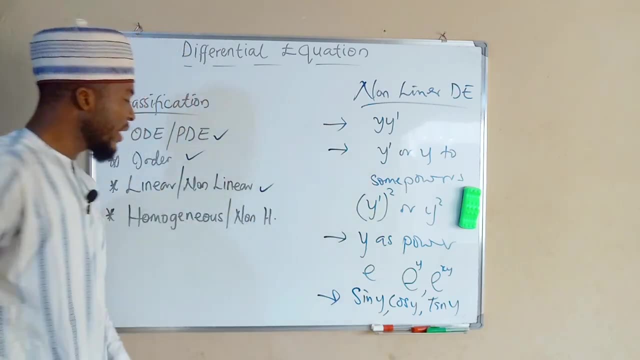 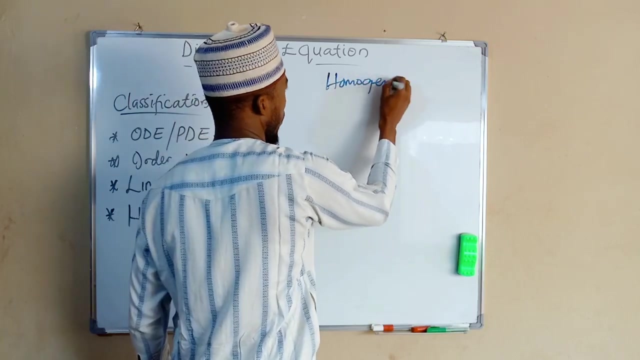 functions. So these are the characteristics of nonlinear differential equation. All other characteristics will fall under linear differential equation. So the last one I want to discuss here is homogeneous or non-homogeneous differential equation, And there are certain ways in which you can determine whether a differential 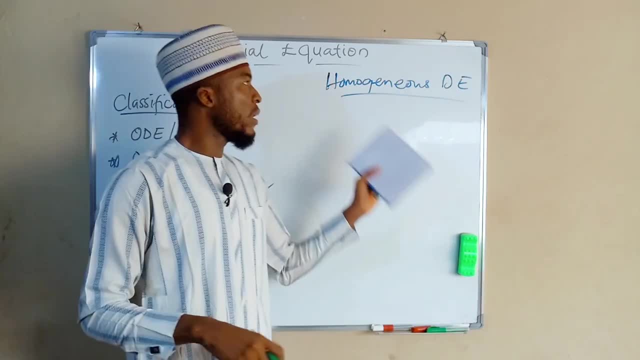 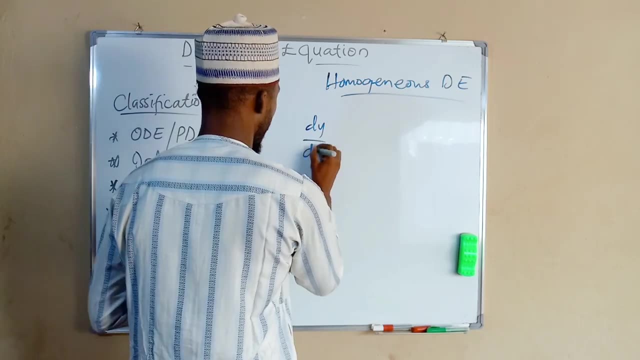 equation is homogeneous or non-homogeneous. In homogeneous differential equation, all terms have the same degree of difference. So if you have a differential equation and you want to have the same degree of difference, For example if we have dy over dx to be equal to x, 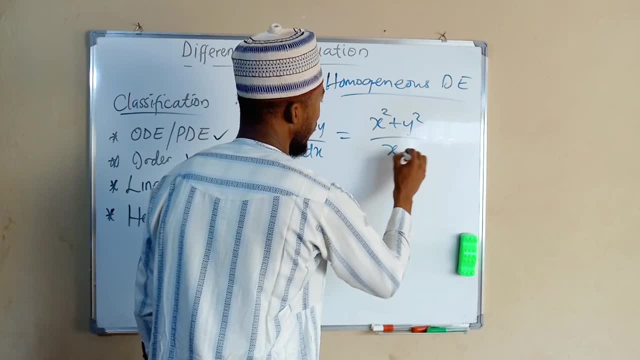 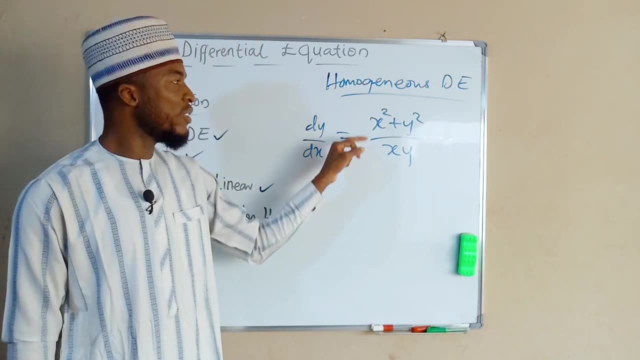 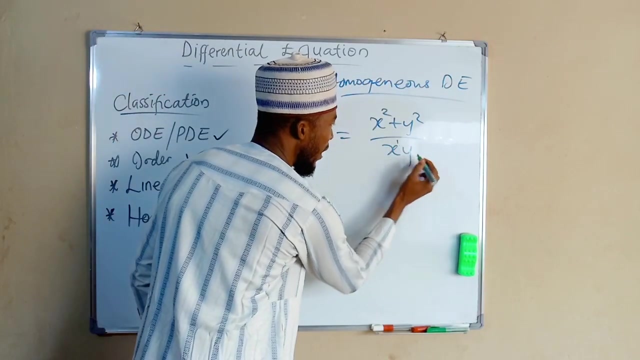 squared plus y, squared over xy. If you can see, all the terms in this differential equation are of the degree 2, because this x is the second power, y is the second power and here we have 1 for x and 1 for y If you combine them. 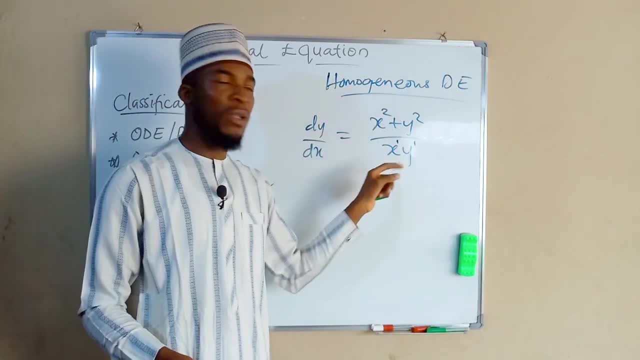 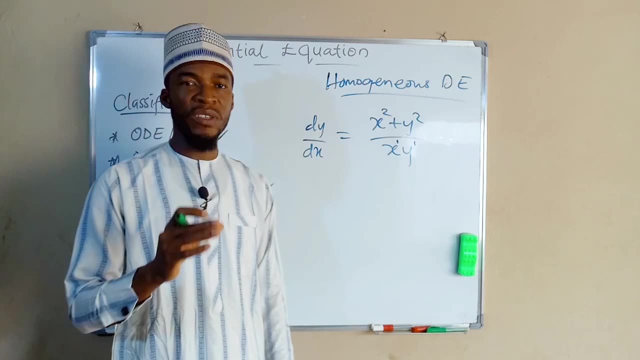 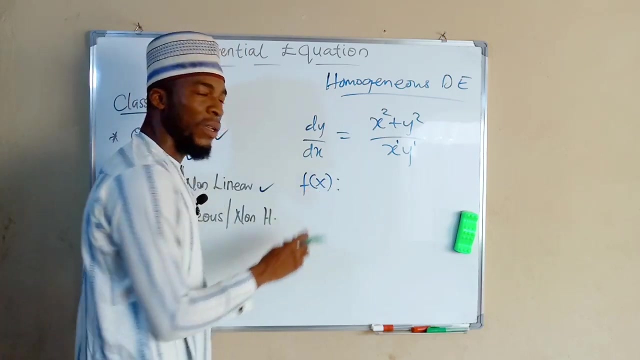 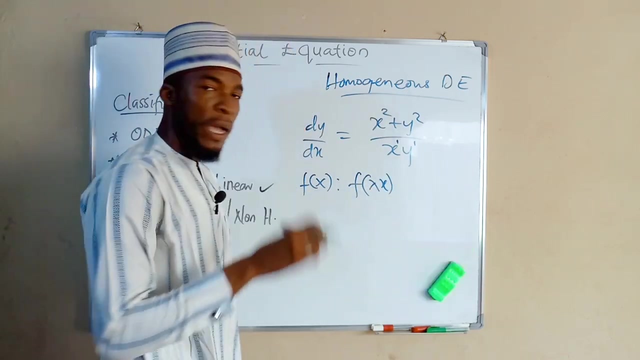 together we have 2.. So all the terms in different, all the terms in that differential equation have the same degree. Another way you can identify a homogeneous differential equation is that when you have a function, say f of x, if you replace that x with some constant times, X, f of maybe lambda X and you 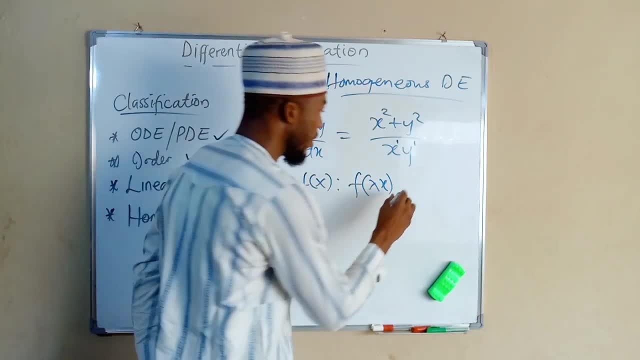 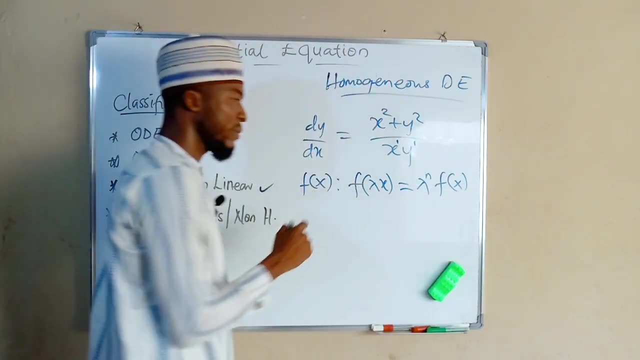 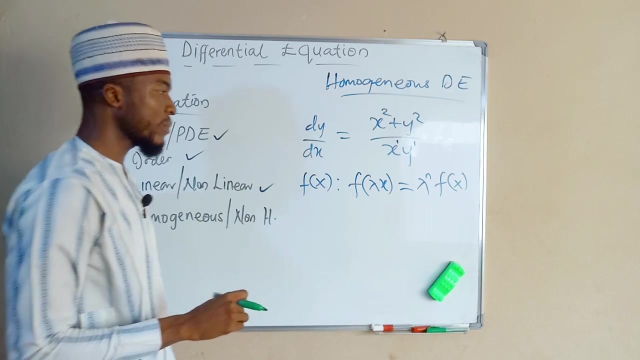 simplify that expression and factor out that lambda you are going to obtain lambda to some power times. the initial function, which is this: If it can be transformed in this form we see it, is homogeneous differential equation where n will determine the order of that differential equation. 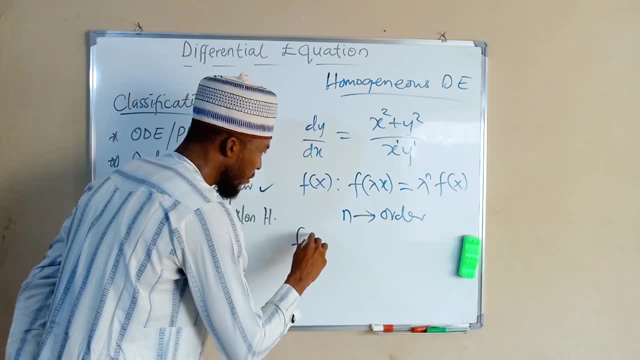 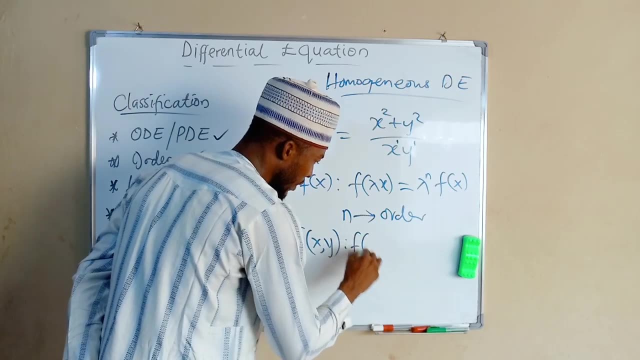 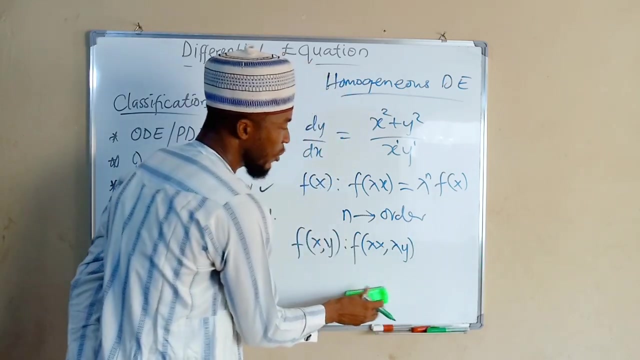 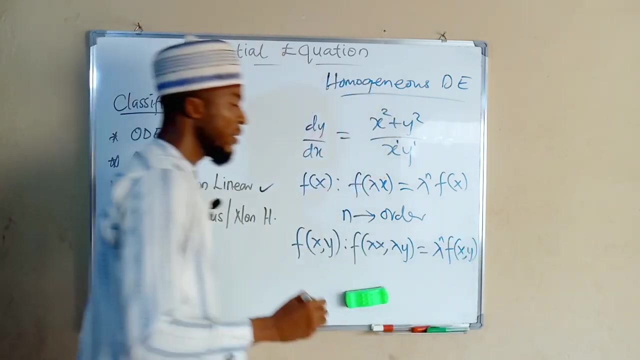 And for multivariable equations, which is maybe x and y, and you replace x with lambda x and y with lambda y, you are still going to obtain lambda to some power of the initial function where n, again, is the order of that differential equation. 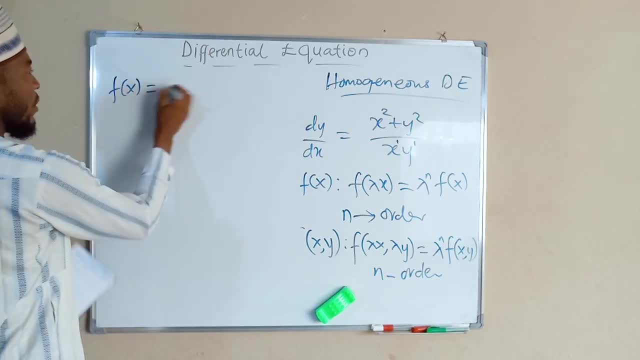 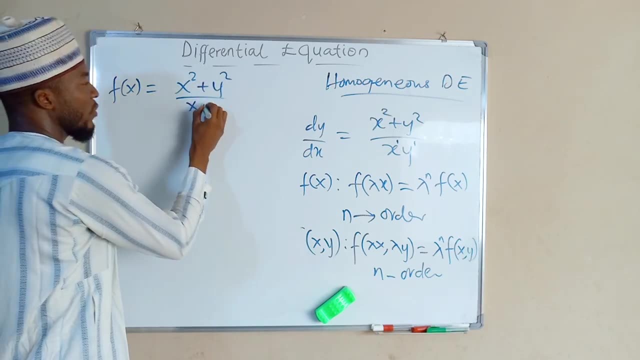 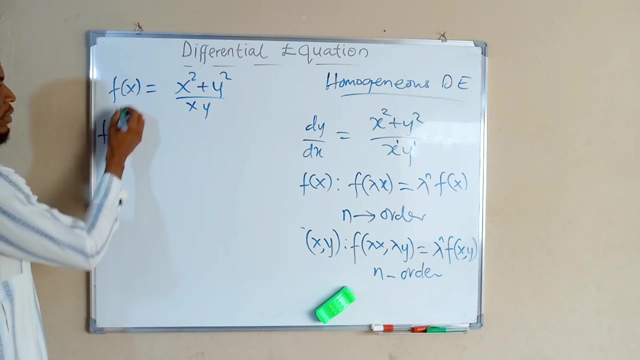 Suppose we have a function x squared plus y squared over xy. We are now going to replace x with lambda x, y with lambda y. So this is a function of x and y. So we are going to replace this with lambda x and lambda y. 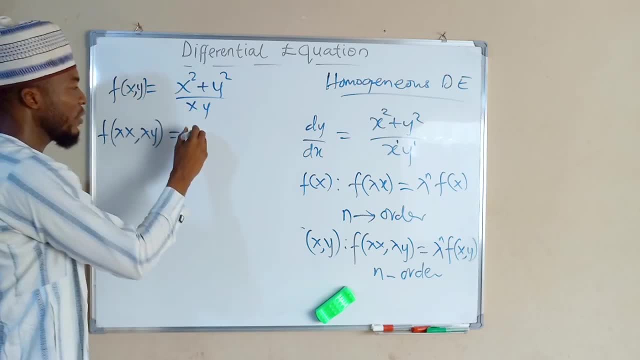 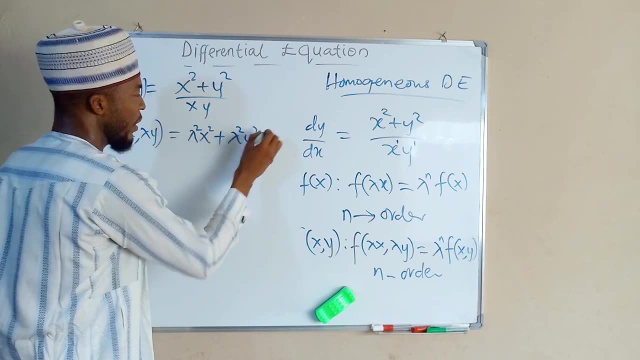 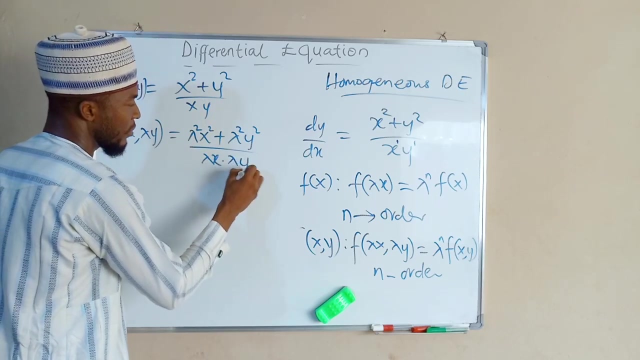 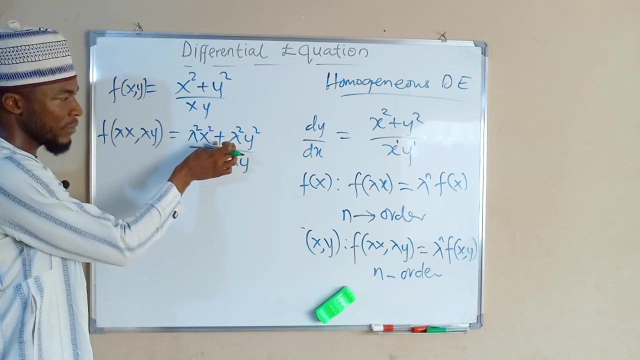 And this will be equal to: if you replace lambda x with x, you are going to get lambda squared, x squared, plus lambda y squared, y squared, And here we have only lambda x times lambda lambda y. From here you can factor out lambda so that we have lambda squared outside. 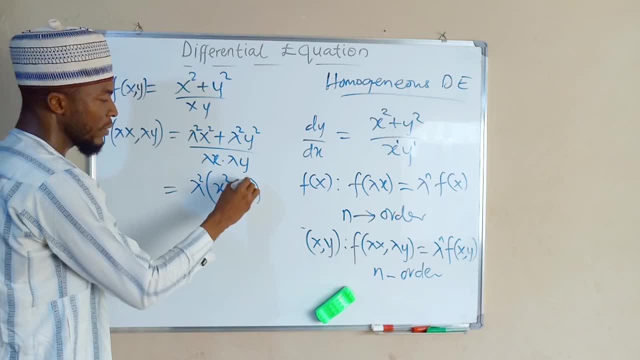 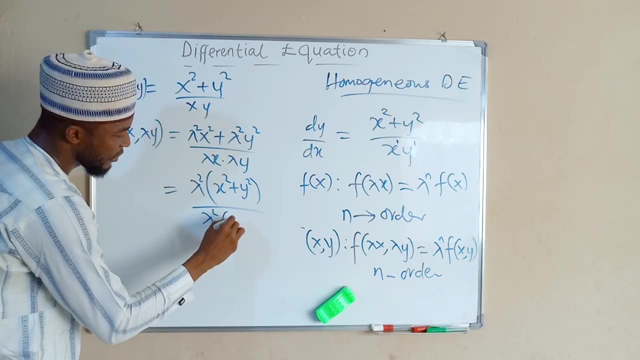 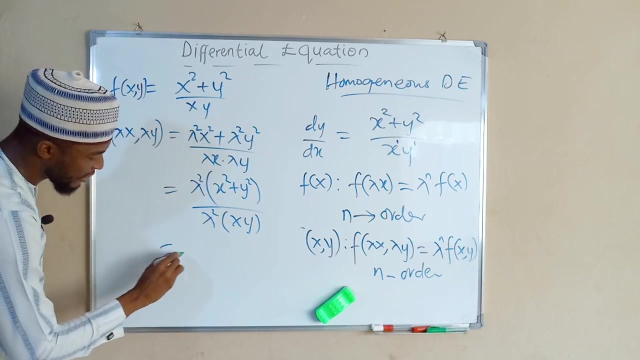 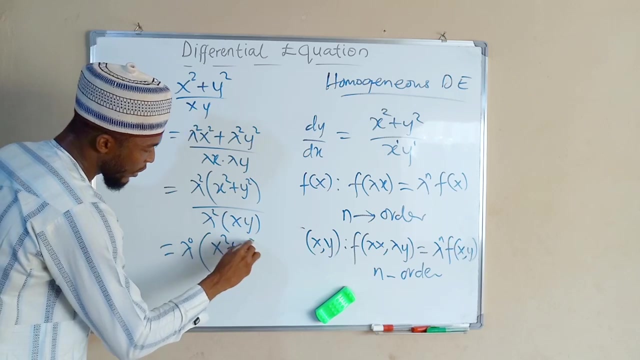 and inside we have only x squared plus y squared, And from the bottom we have lambda times lambda, which is lambda squared times x- y. You can see we have lambda divided by lambda, which is the same thing as lambda power zero of the function, x squared plus y squared over x- y. 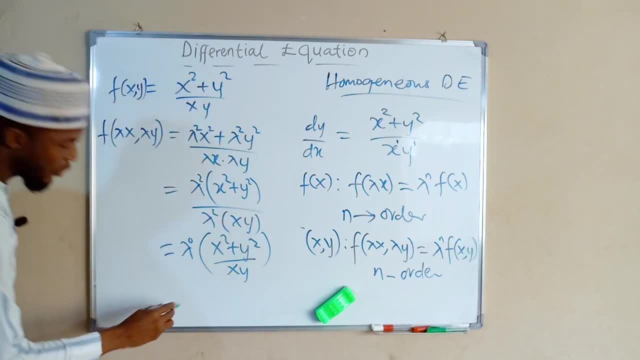 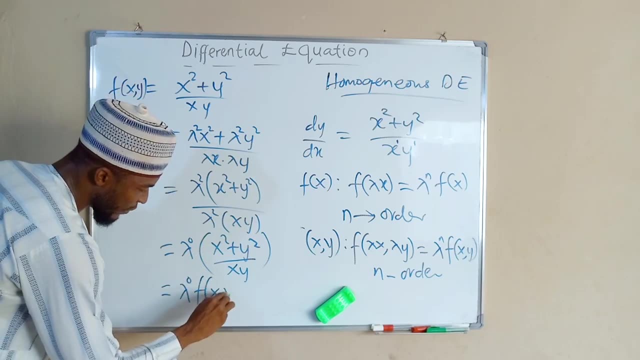 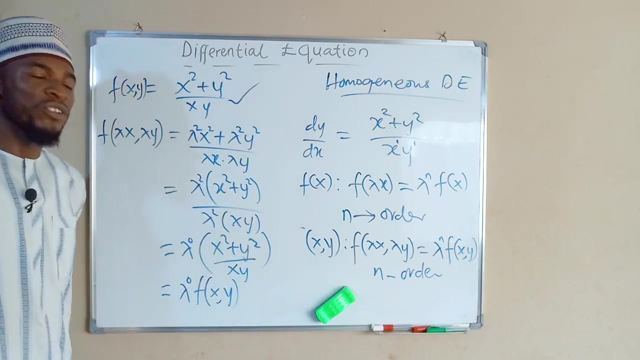 which is the same thing as the initial function. So we say this is equal to lambda power zero of the function, the initial function. So this is what of the degree zero? So we say this is a homogeneous differential equation. Another way you can identify a homogeneous differential equation is: 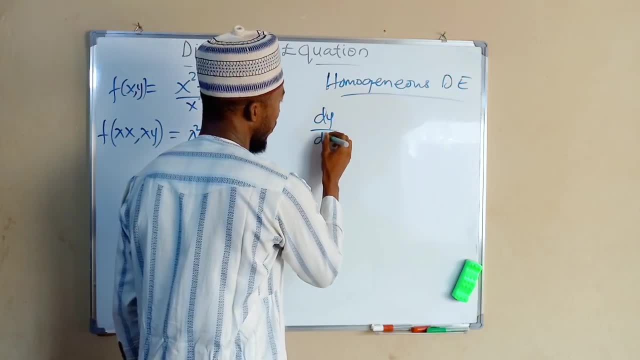 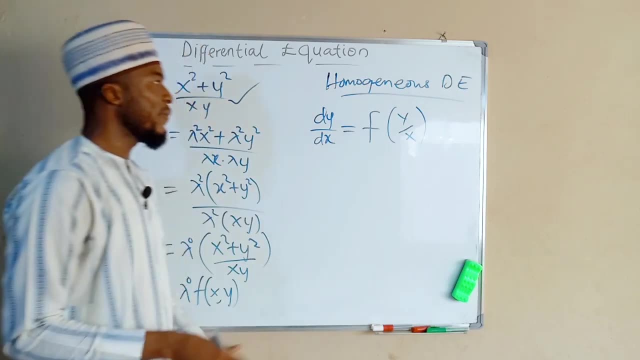 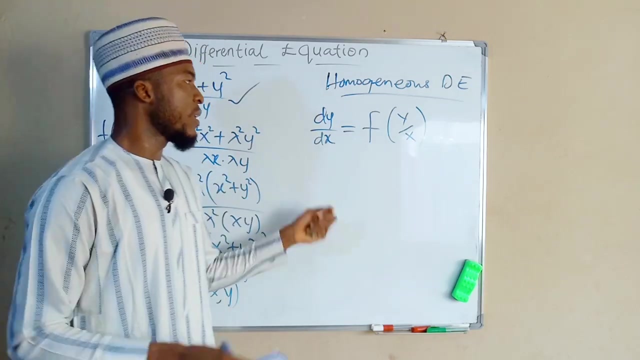 if the derivative in that equation can be written as a function of y over x. If you can transform that function with y over x, we say it is homogeneous differential equation. And the essence of transforming our derivative to this form is if that equation is not the separable type. 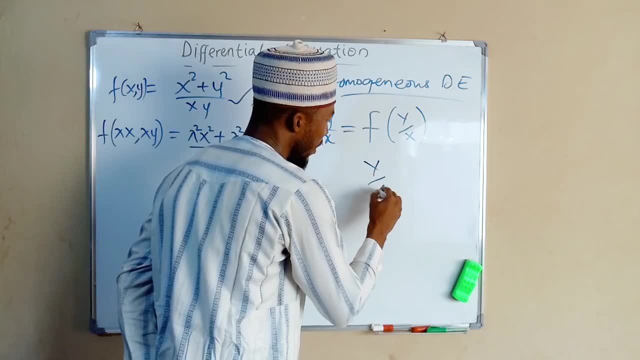 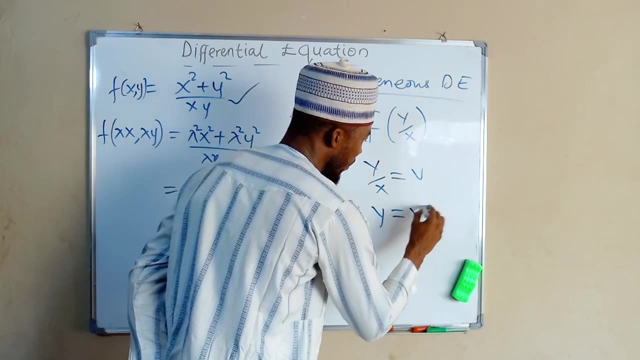 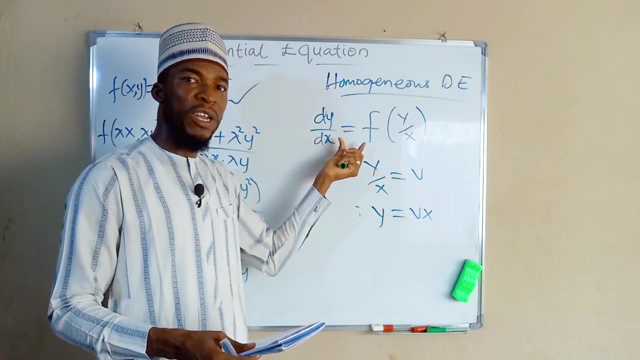 we can replace y over x with v, such that y can be equal to vx. Then we differentiate y with respect to x. By doing so we can transform the initial equation into a separable type. Then we solve for y. This is our example. 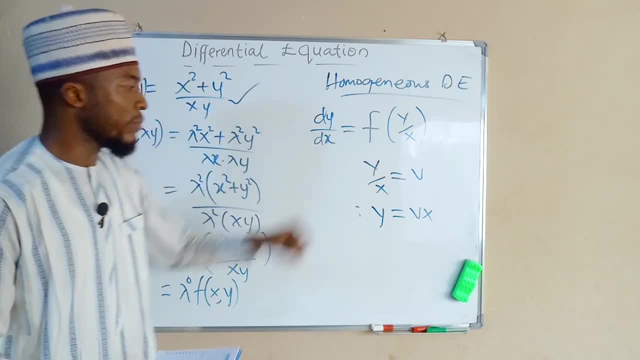 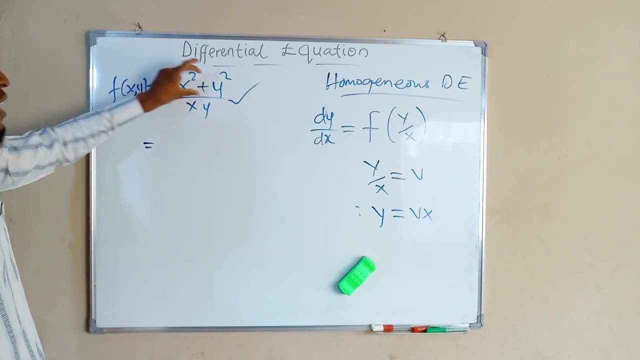 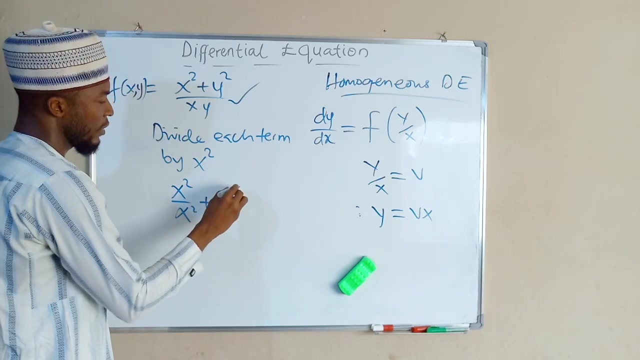 Let's see if we can transform this equation into this form. What we are going to do here. we are going to divide each term by x squared, So we have so that the first term here we have is x squared over x squared, plus y squared over x squared. 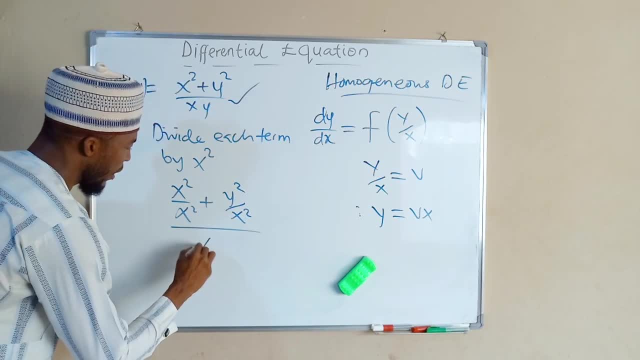 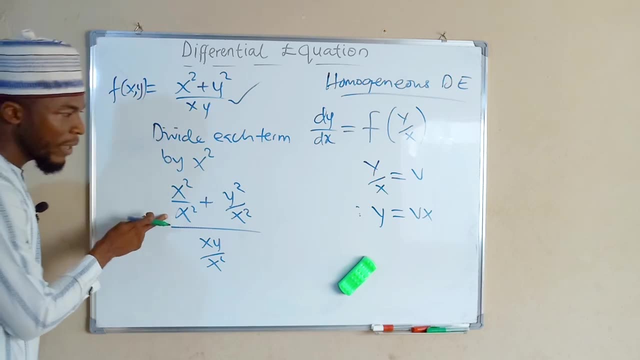 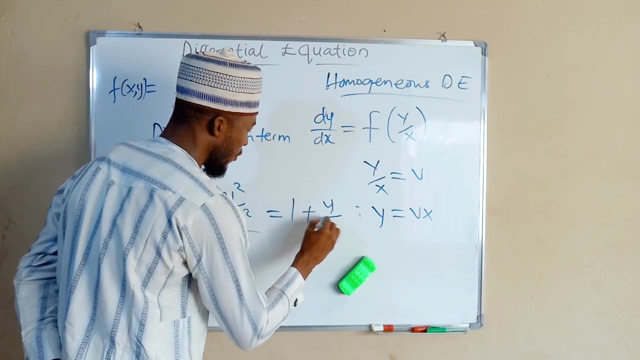 divide by xy over x squared. Now let's simplify: x squared plus x. x squared. divided by x squared, this is equal to 1, plus they have common power, so we can write it as y over x to the power of 2,.